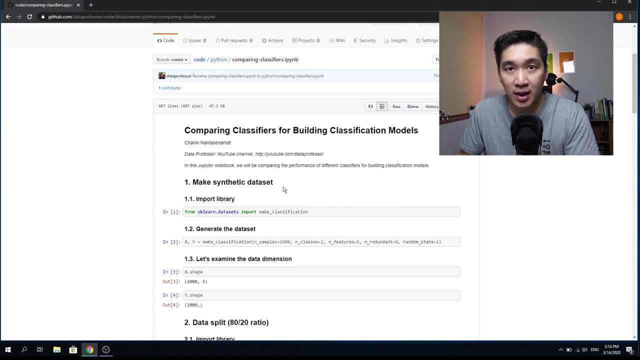 just follow along on the GitHub page here, because it is already in the notebook format And for those of you who would like to follow along, please download a copy by right click on the raw link and then save link as into your computer. So I'm going to save this into. 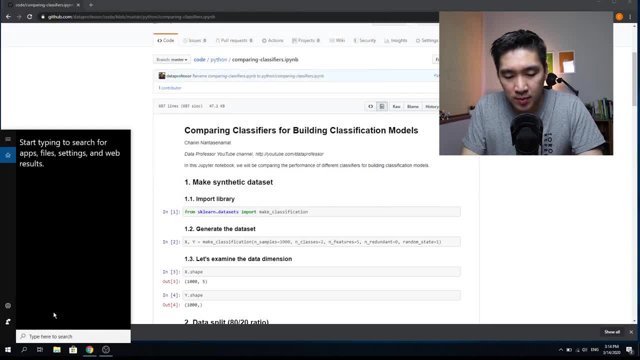 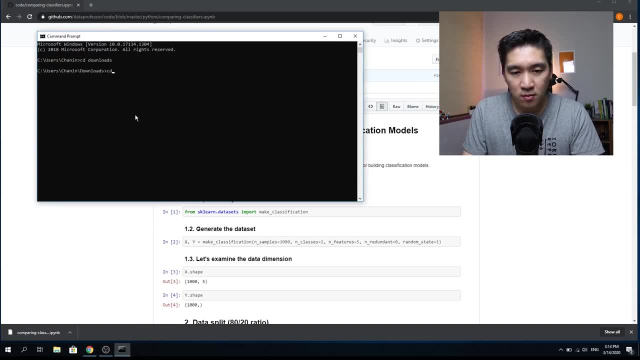 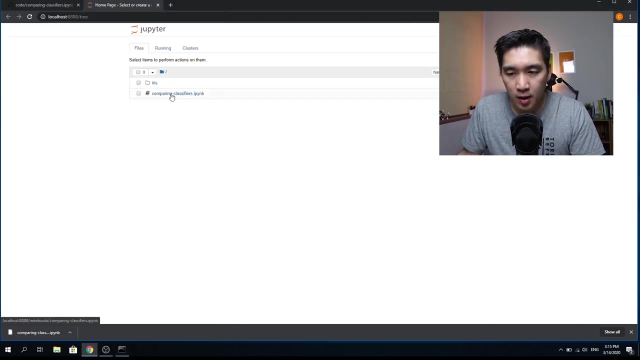 the Python folder. Okay, and then I'm going to open up my command prompt and then head over to the folder. Okay, and then I'm going to activate my working environment in conda and then Jupiter notebook. Okay, and then I'm going to click on the notebook. 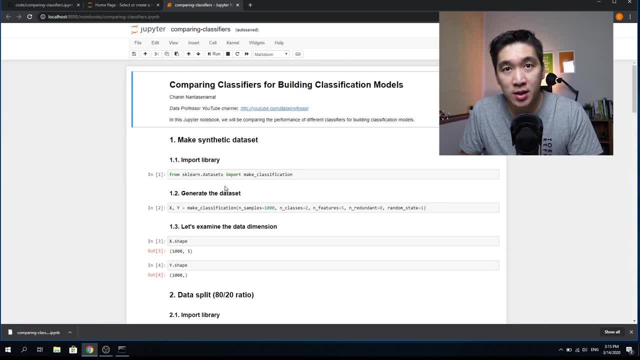 Okay, so here let's begin. So the first thing that we want to do is to create a synthetic data set, And in order to do that, we're going to use the make classification function of the scikit learn package. So to run. 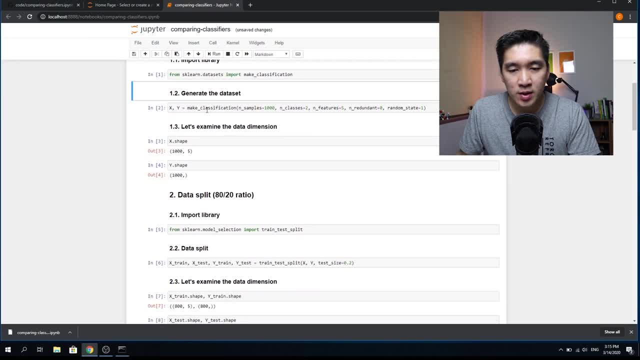 this: go ahead and shift, enter, And then we're going to generate the synthetic data set by using this make classification, And then we're going to assign it to the x and y variable, which will be newly generated as a result of this function, And so the input argument that we're going to use here. 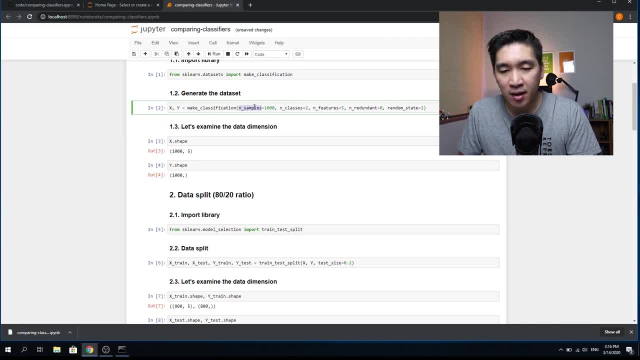 is, we're going to create a synthetic data set comprising of 1000 samples. So for n underscore samples we're going to have it assign a value of 1000.. And for n underscore classes, we're going to assign a value of two, because we're going to create two classes for this data set and n underscore. 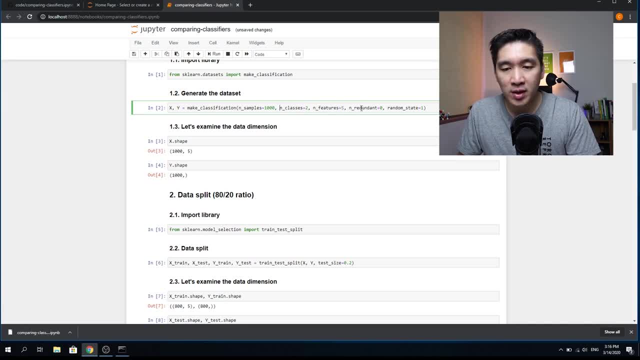 features. we're going to have five, So n underscore redundant. we're going to have it zero, And then we're going to assign the random underscore state To be one. okay for reproducibility. So let's go ahead and run this cell. Okay, so let's examine. 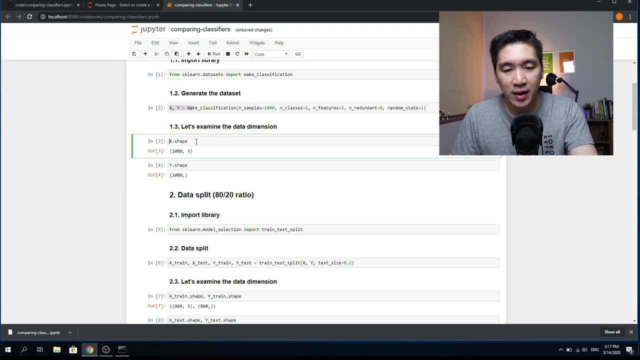 the shape of the newly generated variables. So x dot shape will give us 1000 rows, which is the first value, and a second value correspond to five column, which is the number of features here which we have already assigned a value of five. and then the y dot shape will give us 1000, which 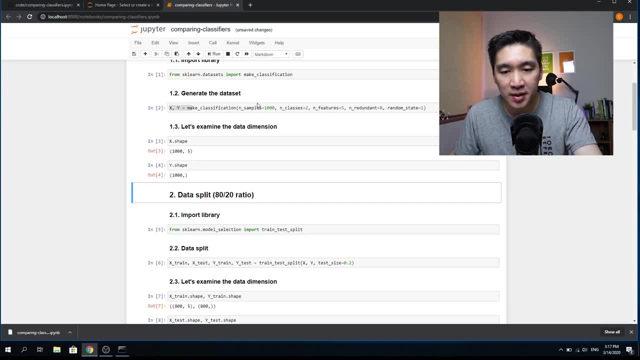 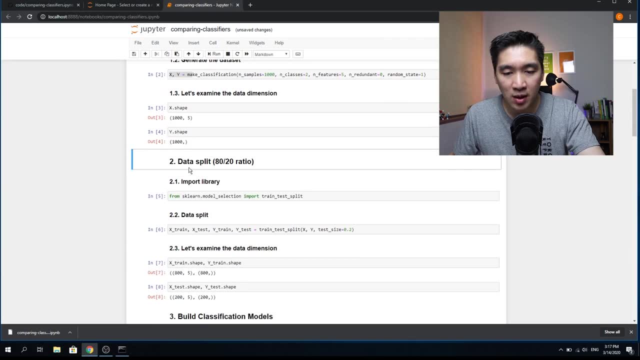 will be the same dimension here, because there are 1000 samples and no value follow this one. so it means that there is one column, which is the y class label. So the next step that we're going to do is we're going to split the data into 8020.. So we're going to import the library, particularly. 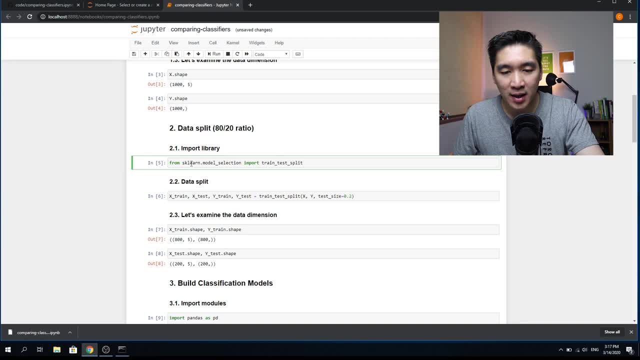 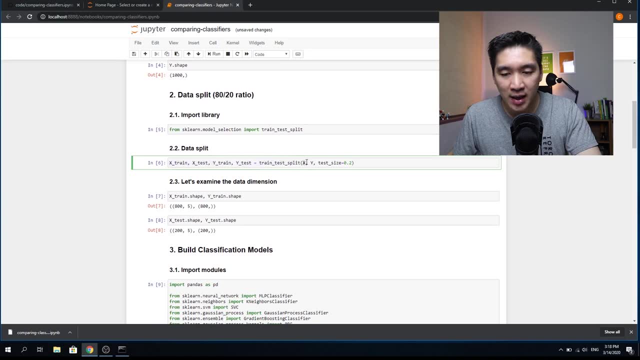 we're going to use the train test split from the scikit learn package, So go ahead and run that and the data split will be performed here using this train test split, And it will take us input the x and y variables, which corresponds to the five input features, and the class label and test size. 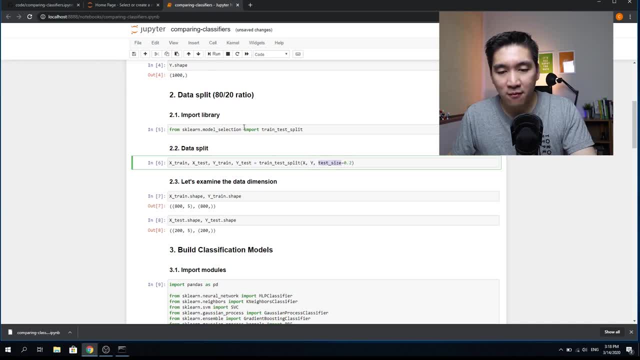 0.2,, which is the 20%, And then the 80% will be for the train. And so here we will generate four variables concurrently and it will comprise of x train, x test, y train and y test, So the two x here. 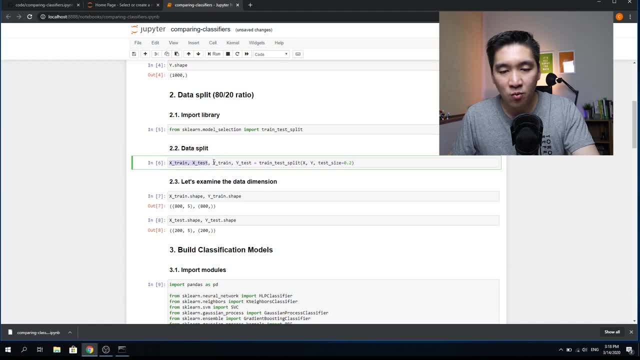 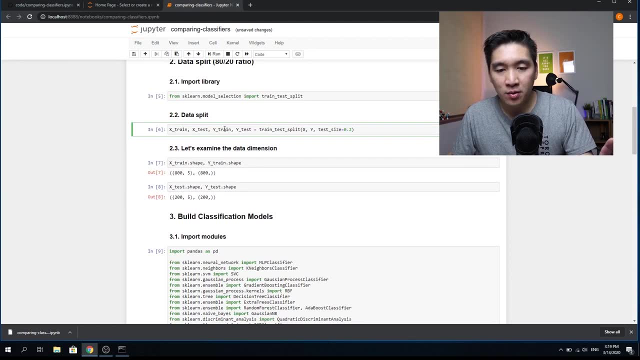 are the input features, the five input features and the y train and y tests. are the class labels, right? Okay, so the x train and the y train will be used to generate the machine learning model And after we have done that, we're going to apply the 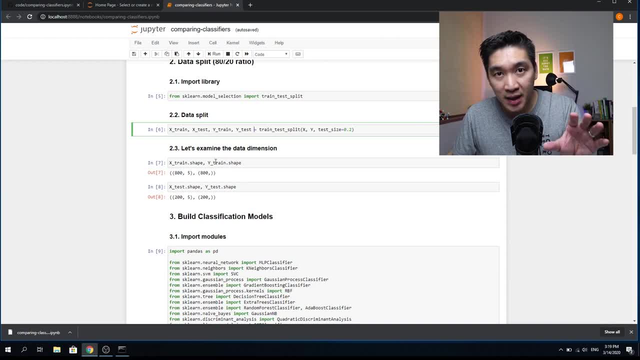 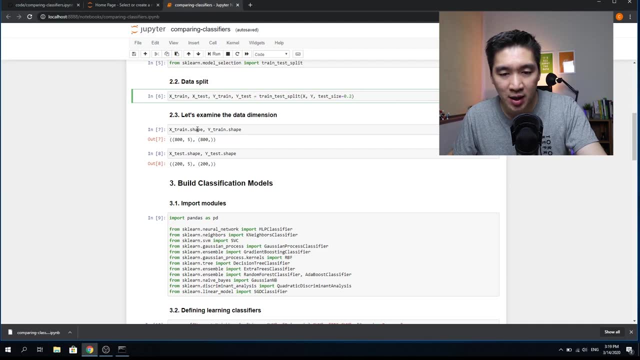 machine learning model to make a prediction, which we will be using the x test. So we're going to mention that below. So let's examine the data dimension. So x underscore train dot shape will give us 800 by five, because there are 800 samples And because 80% of 1000 is 800, and y train dot. 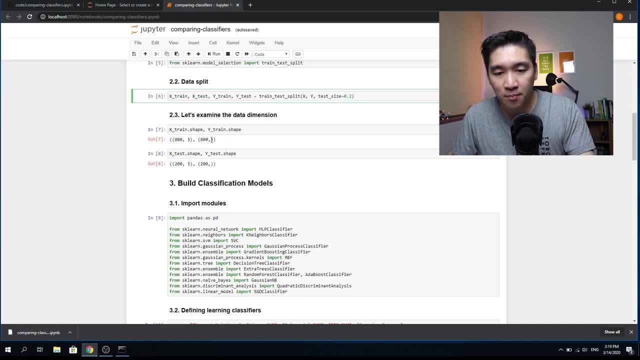 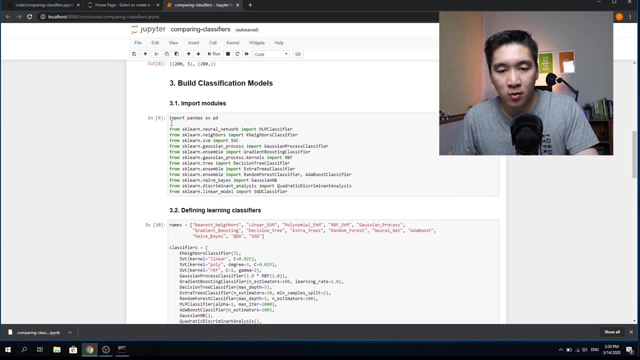 shape will give us 800 rows and one column. X test dot shape will give us 205, which corresponds to 200 samples and five columns. Tesla shape will give us 200.. So the fun part is right here. So we're going to import all of the 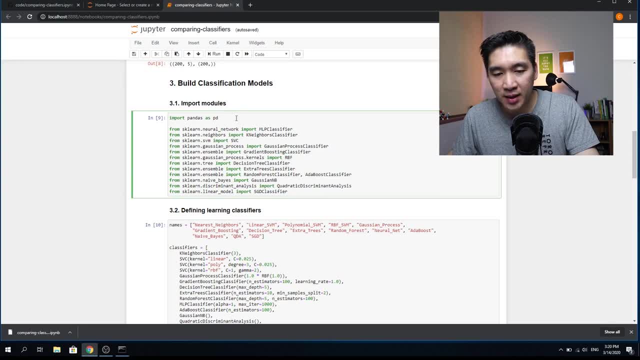 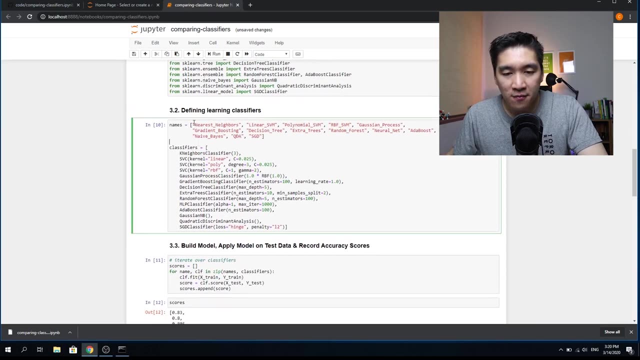 modules. So the first one will be pandas, SPD, for the subsequent generation of the data frame of the results, And then the big chunk of code here will be all of the machine learning algorithms that we're going to use. So we're going to run that And the names of all of the machine learning. 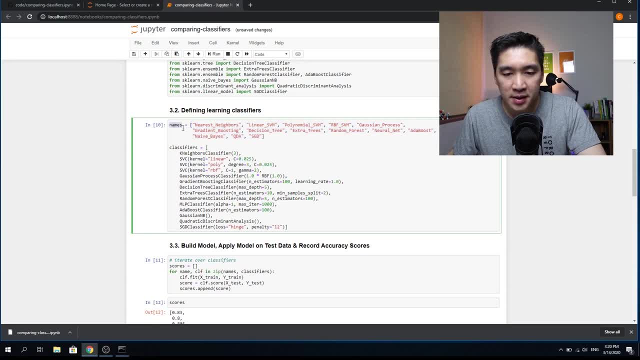 algorithms are shown here in this names list, And then the classifiers will contain a list of all of the machine learning algorithms that we're going to use. So here we're going to use the basic input for the algorithms. So in a future video we're probably going to cover about how you can optimize. 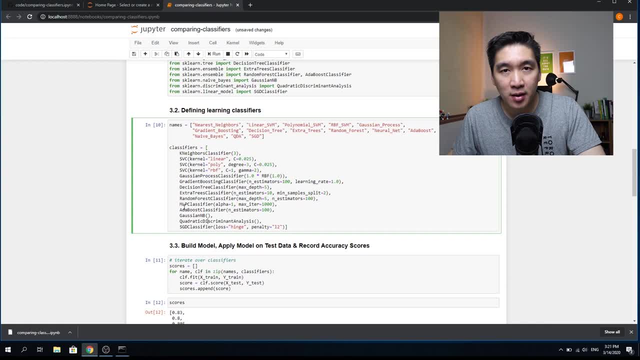 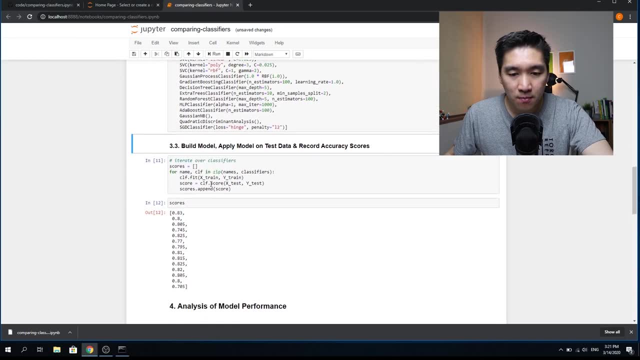 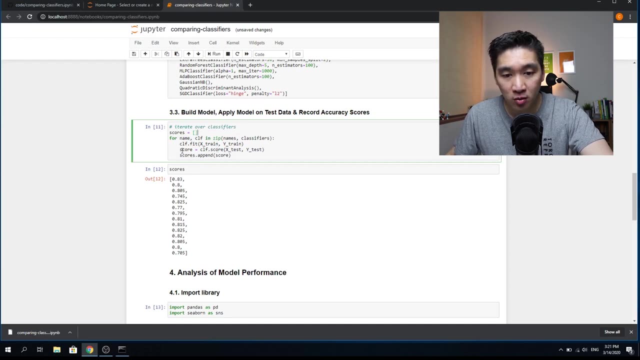 these hyper parameters in an automated way. So stay tuned for that one. But today we're just going to use the default values, So go ahead and run that line, Okay. so now we're going to iterate the construction of the machine learning models one by one in a for loop. So 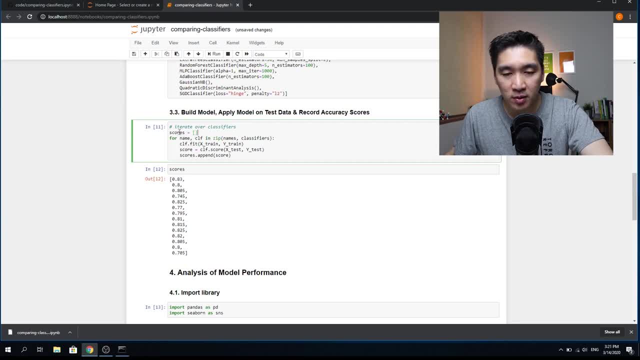 firstly, we're going to generate a empty scores variable where the model will be generated, and then the scores of the model will be calculated, And for each iteration, which will correspond to the construction of one machine learning model out of the 14 machine. 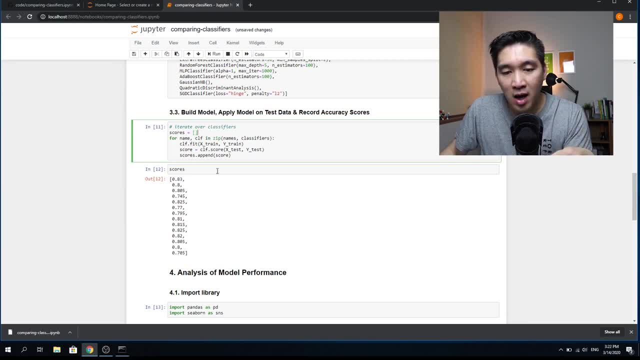 learning models and for each of the machine learning model it will output the score and each score be appended to the scores variable. So, because there are 14 machine learning algorithms, the for loop will occur for 14 times And for each time it will output a score: the accuracy score. 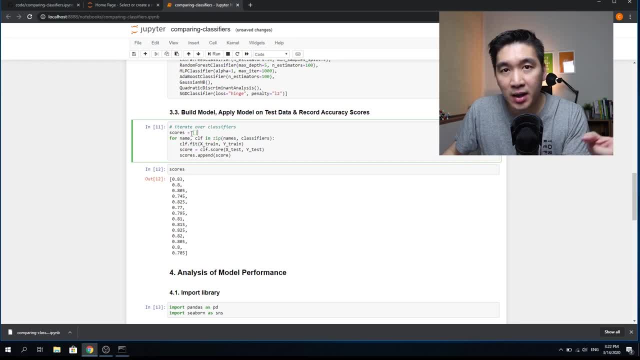 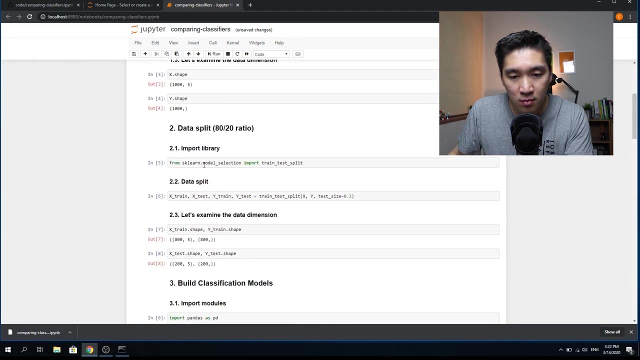 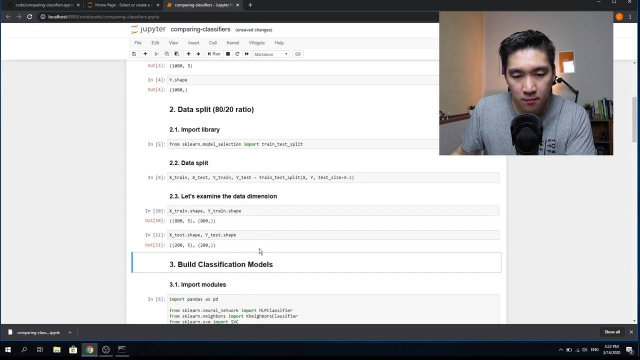 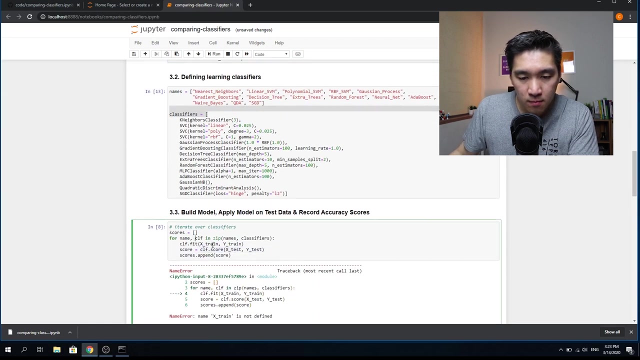 and add that to the scores variable, And because it's going to loop this over and over for 14 times. therefore, the scores variable will be a list of 14 accuracy score values, So let's go ahead and run that. Okay, so we haven't run this yet, right? Do it again. Okay, so the model building will. 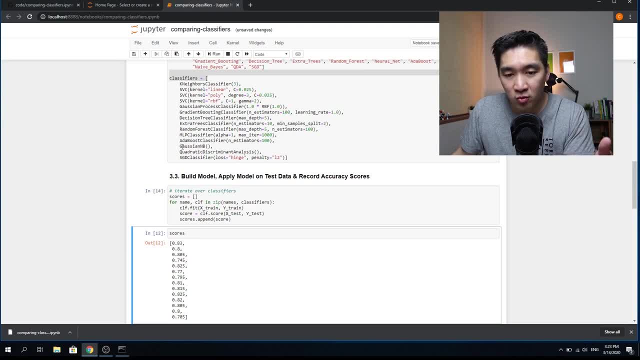 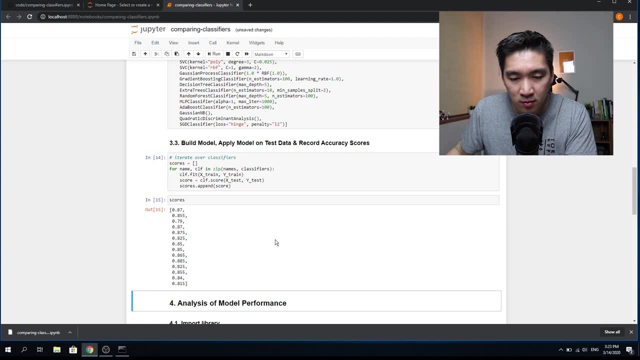 take some time because it is looping over 14 algorithms. Okay, so model building is finished And then we're gonna just type in scores so that we see the value of this variable. So the accuracy score of the 14 machine learning models are shown here. So the 14 machine 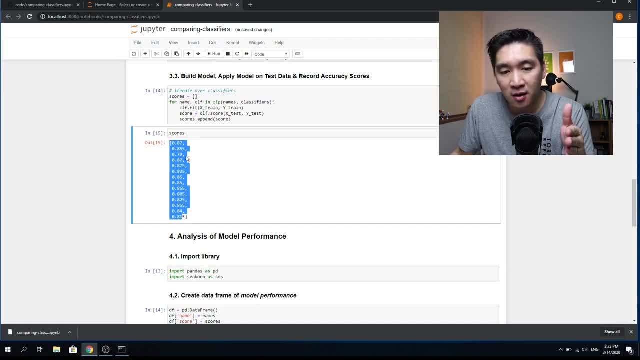 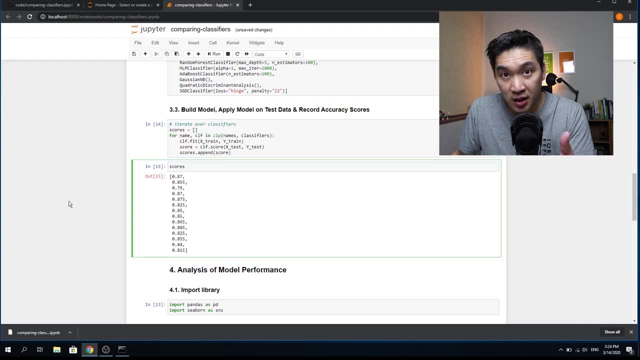 learning model gave a accuracy score in the range of 0.79 and 0.885.. So maybe you're wondering that the score list here is good, it's informative, but it's a bit too plain. So let's see if we can. 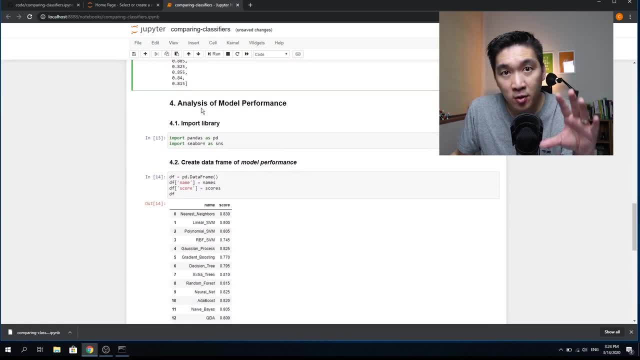 spice it up a bit. So this is the purpose of the fourth section here, So analysis of the model performance. Okay, so the first part: we are going to import the library, So we're going to use the pandas and we're going to use seaborne, And so then we're going to create a data frame of the result. 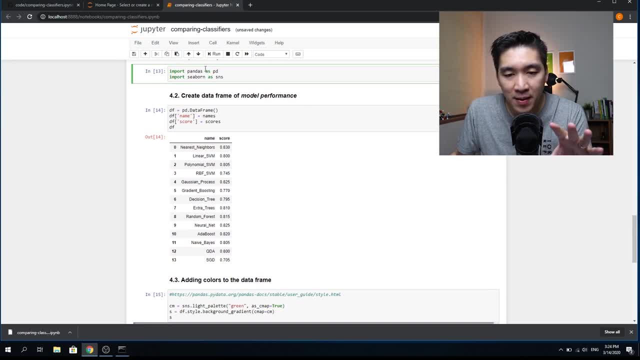 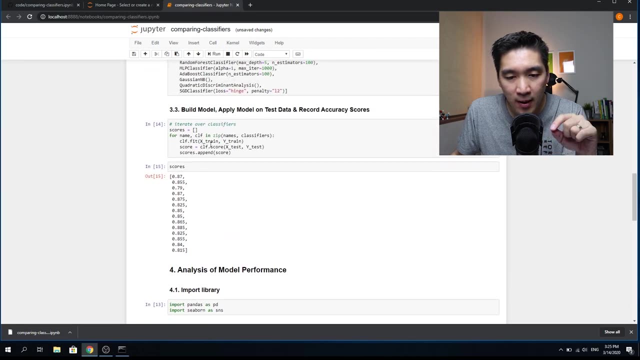 So DF equals to PD, which is using the pandas function dot data frame. So this will create an empty data frame and then DF bracket And then we're going to use single quotation name equal to names And the names here will coming from here. The names right here: the name of the: 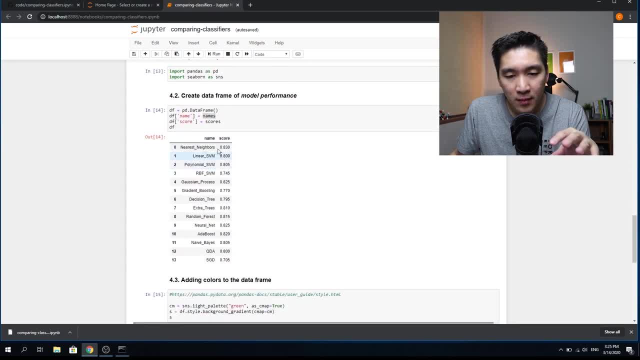 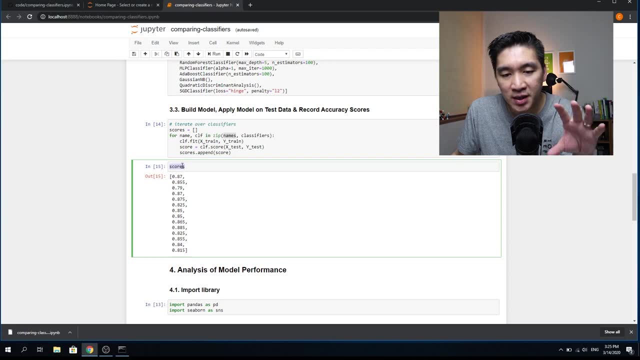 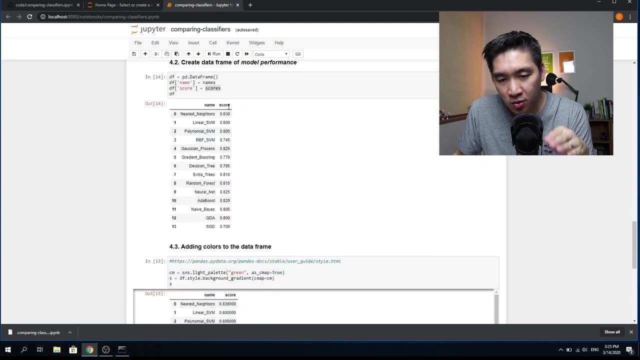 machine learning classifier And then the scores will come from the scores. So the scores variable will contain the 14 accuracy score from the 14 machine learning algorithms. So here we're going to use name and score. So we have the name of the 14 machine learning algorithms and the 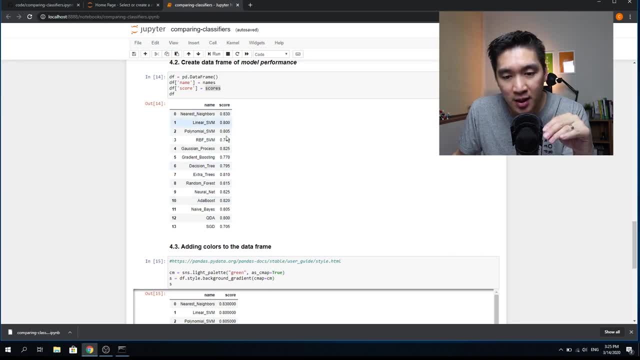 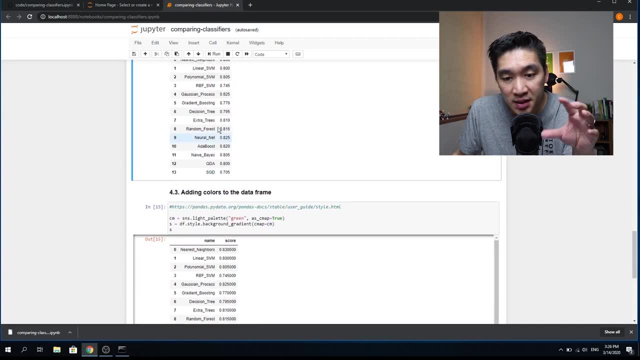 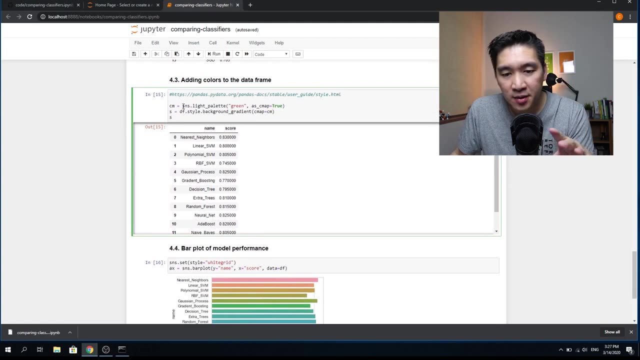 corresponding accuracy score. So this looks much better than the previous list that we can see here. So maybe you're wondering: okay, this is good, but can I have it a bit better? Okay, so let's have a look here. So what about we add some color to this? Okay, so here we're going to. 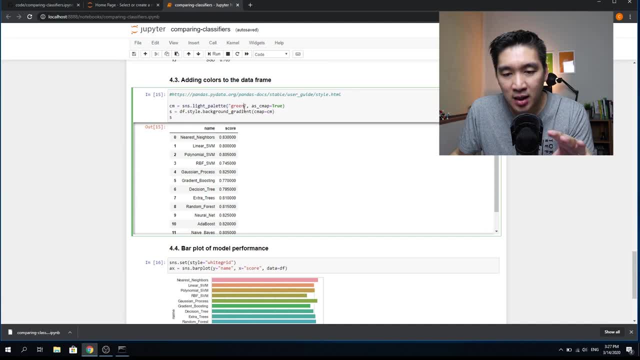 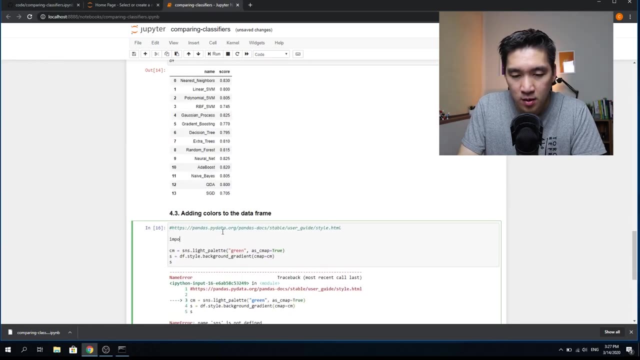 use the seaborne and light palette function and the color is green, So feel free to change this to other color that you like, And we're going to style the background as you can see here using this function: style background gradient. And okay, so I have to import seaborne. 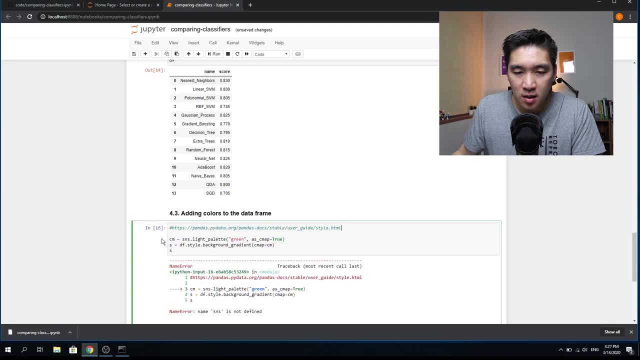 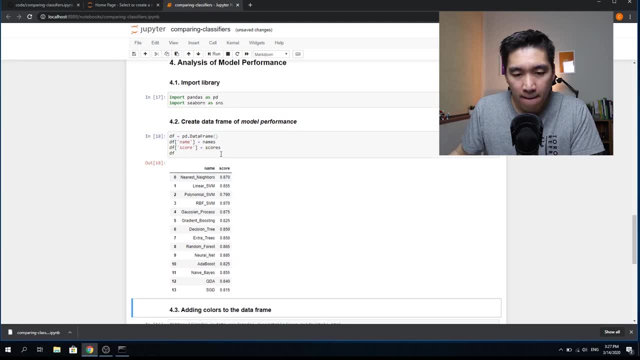 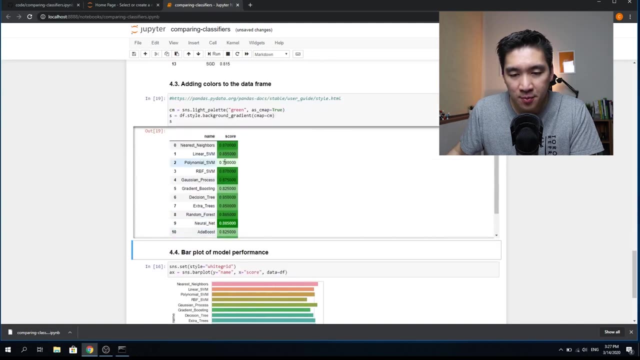 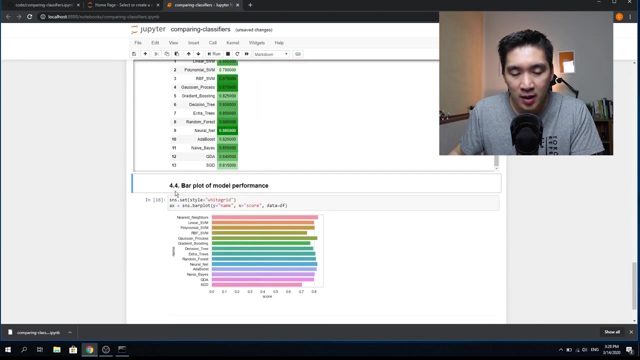 So let me put it up here. Oh, I already have it, Okay, but I didn't run it, So let's run it. Okay, there you go. So you can see that the model with the least performance will have lighter shade of green and the best performance will have darker shade of green. here, And let's have a look. 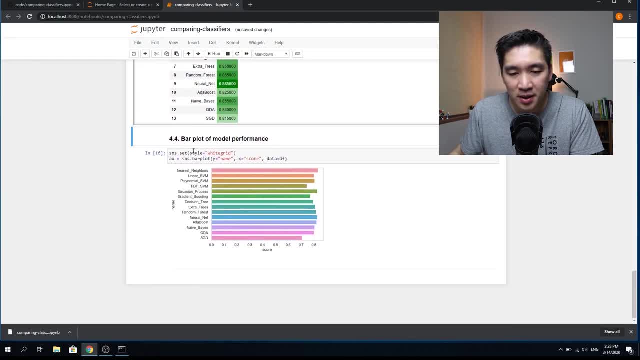 in another way. So if we make bar plot of the model performance, so let's say that we want to to have the background to be white, And then we're going to create a simple bar plot. So the y axis will be the name of the machine learning algorithms and the x axis will be the accuracy. 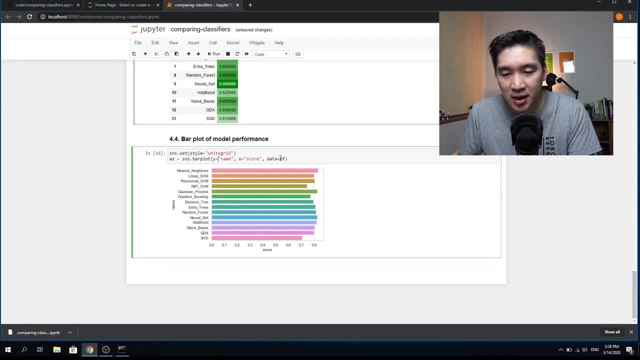 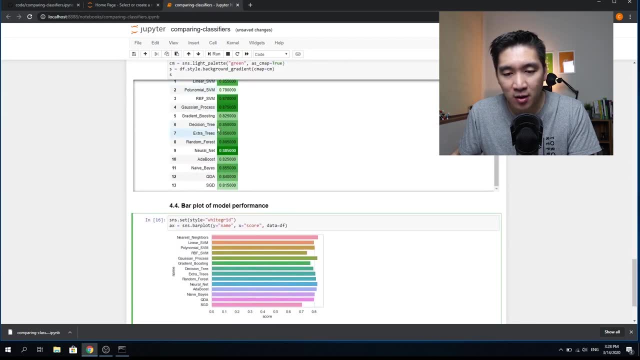 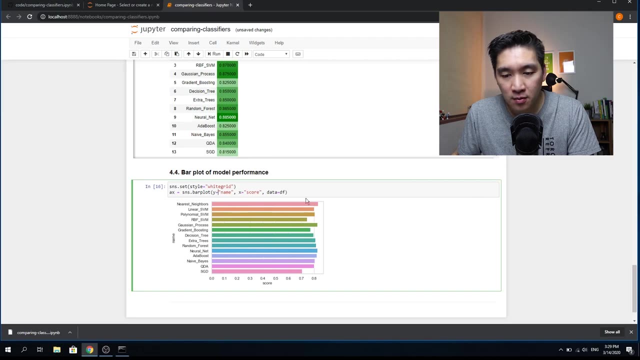 score, And so here we're going to specify that the input data is coming from the DF dataframe, And so this is a graphical view of the same data that we have here. So choose whichever one that you like, Or you can even use both. So feel free to play around with this code, And we're going to